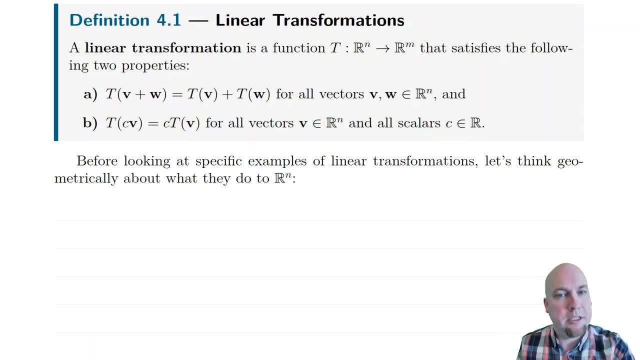 Okay, but it's not just any function sending n dimensional space to m dimensional space. It's got to satisfy these extra two properties down here, these properties that I've called a and b, And basically what these properties say is: the function plays well with the standard. 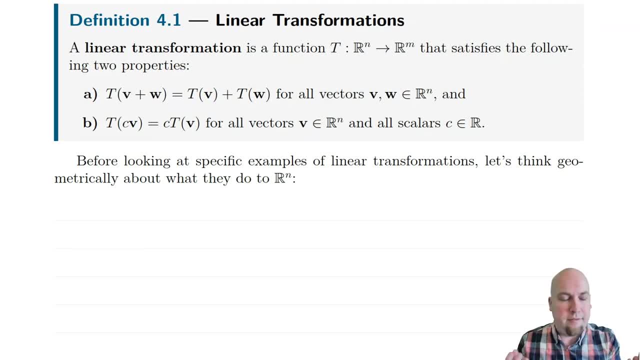 linear algebra operations. Okay, with the standard operations on vectors. Remember, we've got vector addition and we've got scalar multiplication and well, basically, the two properties of linear transformations relate to those two operations. Okay, so, let's look at this. Okay so, let's look at this. Okay so, let's look at this. Okay so. 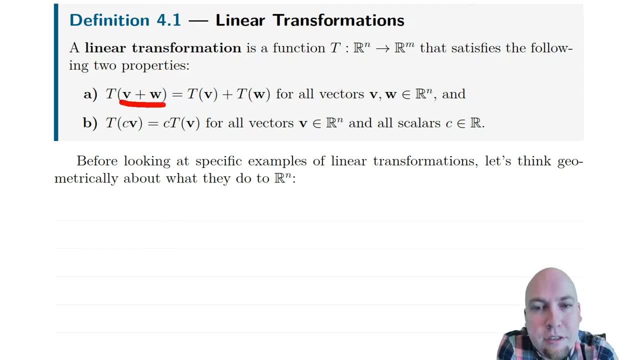 the first property here, property a, says that if you add two vectors and then apply the linear transformation to that sum, you get the same thing as if you apply the linear transformation to the vectors and then add them up, In other words, in a sense like applying the linear. 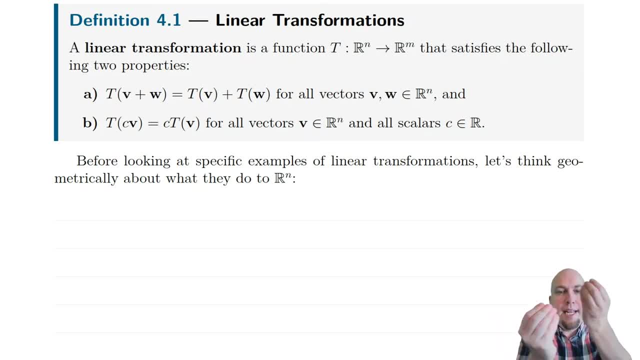 transformation. it kind of commutes with vector addition. You can do them in either order and you're going to get the same answer. Okay, then property b is the analogous thing for scalar multiplication. You can scale or multiply and then apply t, or you can. 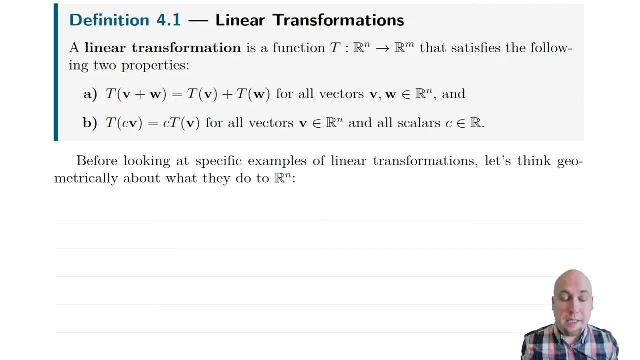 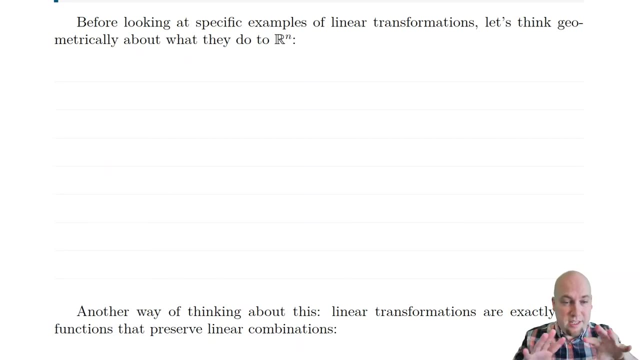 apply t and then scalar multiple and then scalar multiply, and you'll get the same answer either way. You can do it in either order. In other words, you can pull scalars out of the function. Okay, all right. so before we look at specific examples of linear transformations and do things, 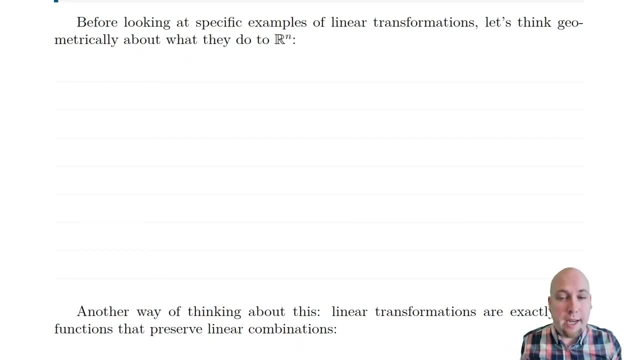 with them. I want to sort of draw a geometric picture of what they're doing. Okay, and I'm going to convince you of this geometric picture, hopefully at least by the end of today's lecture. Okay, but for now I'm just going to draw it and then I'll try to convince you of it later. 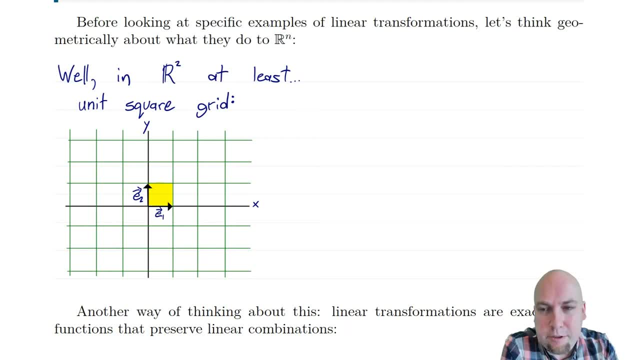 So let's draw a picture. well, in two dimensions, because I can't really draw pictures in higher dimensions. Yeah, anyway, all right. so in two dimensions, let's start off by drawing two dimensional space and I'm going to overlay a grid, a unit square grid on two-dimensional space. just. 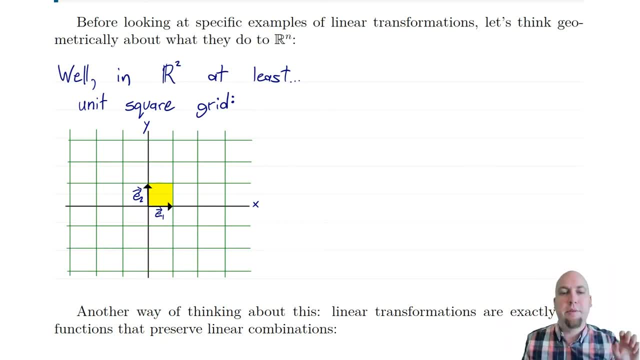 to make it a little bit easier to visualize after I apply the linear transformation to it. Okay, so here's two-dimensional space. I've drawn this unit square grid here and I've also highlighted one particular square here, and that is the square that has e1 and e2 as its sides. Remember, these are the 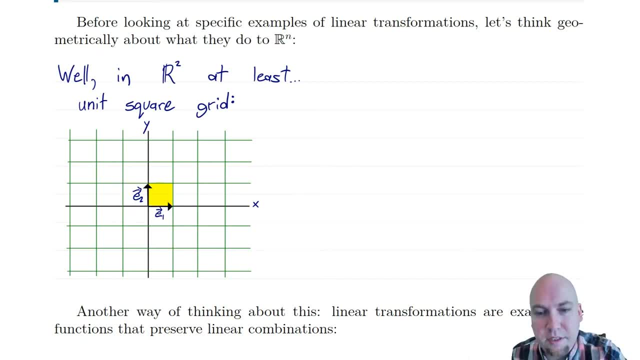 squares. This e1 is 1, 0 and e2 is 0, 1, so it just points up a distance of 1.. And then I sort of highlight in yellow here sort of that first square in the positive quadrant. Okay now, if I apply a, 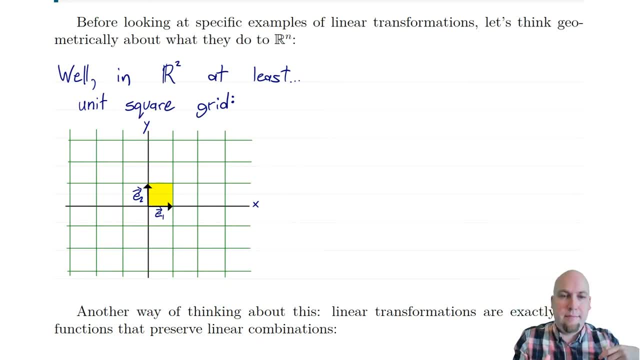 linear transformation to this space. I'd like to know what space looks like after I apply this linear transformation And, in particular, I'm going to start off- I'm going to focus on what it does to e1 and e2.. Okay, and in a sense, I don't know what it does to e1 and e2, right, I mean, it's just. 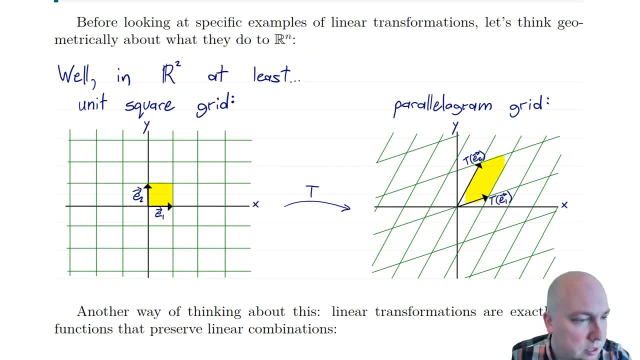 some function So it can send e1 wherever it wants to- let's just imagine that it was sent over here- and it can similarly send e2 wherever it wants to. Okay, so it can send those two vectors to anywhere. But then the point is: once you know what happens to e1 and e2, once I know, oh, 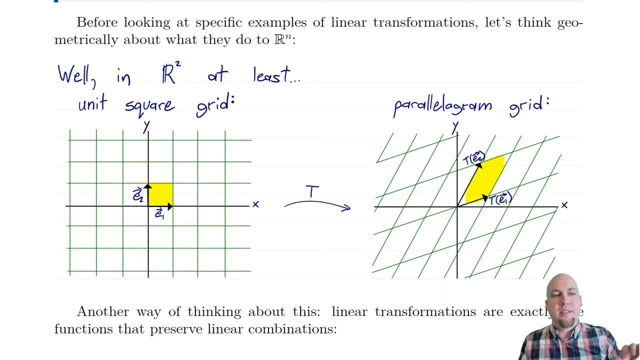 here's t of e1 and oh, here's t of e2, then you know what happens everywhere else. Because what linear transformations do is they send this unit square grid into some parallelogram grid. Okay, that parallelogram, it just has sides t of e1 and t of e2.. So in other words, this linear 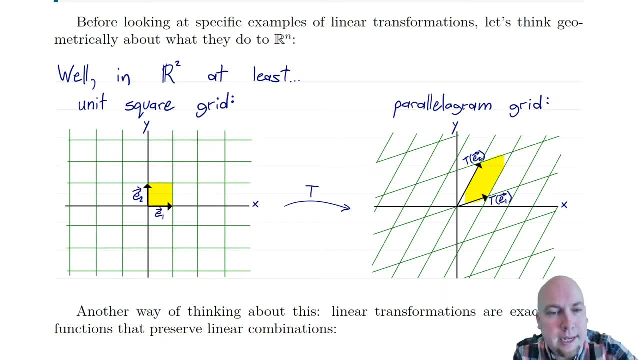 transformation. it's just taking this square grid here and sort of stretching it. Okay, it's sort of stretching and deforming it into a parallelogram grid. And you know what parallelogram grid gets made? Well, that's just determined by these two vectors here that you have to compute. 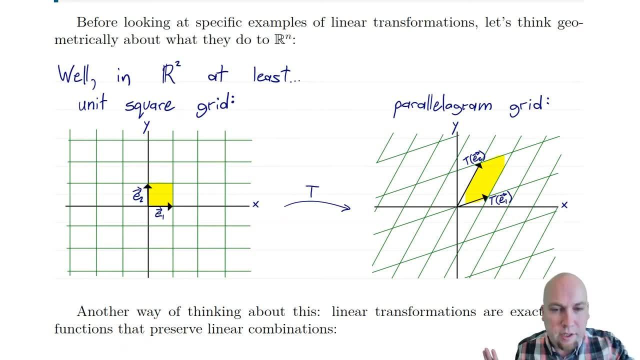 Okay. but the point is, once you know what happens to those two vectors, you know everything. So, for example, then if I give you another vector, if I say, okay, now I'm interested in what happens to this vector v here, Okay, well, then what you can do is you sort of notice that oh, 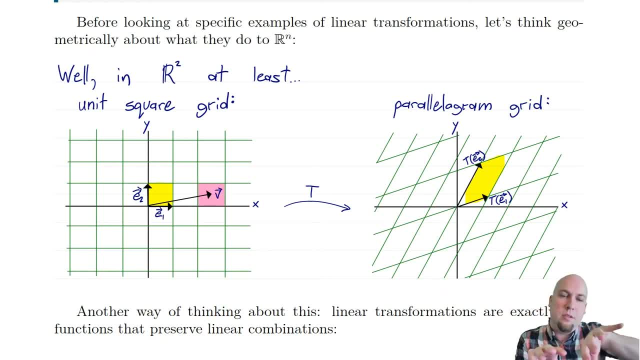 okay, hey, it's, it's over in this pink square over here. that's sort of three squares in the e1 direction and just one square up in the e2 direction. Then, well, this vector v, it's going to get sent over three squares, or three parallelograms now in the t of e1 direction and one square in the 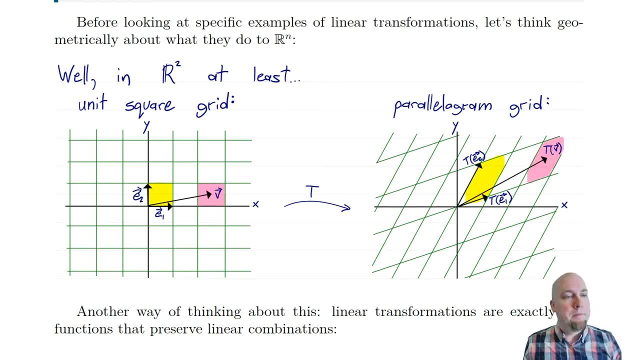 t of e2 direction, So it's going to get sent over there, Okay. so it just sort of stretches and sort of in the same way It's very uniform in this sense. Okay, we'll come back to that in a little bit, once I've hopefully, maybe actually convinced you that this picture is true. 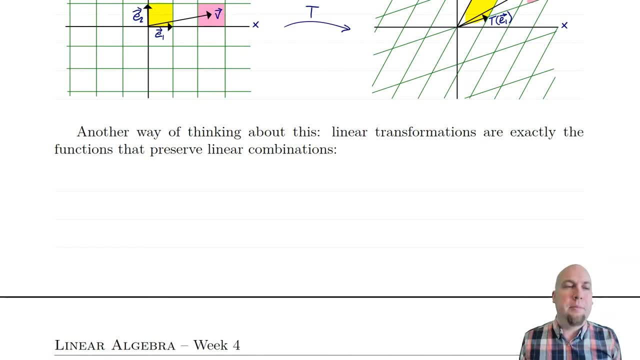 But for now I want to sort of give you another way of thinking about linear transformations, and that is well. they were defined as functions that preserve vector addition and scalar multiplication. And remember, if you combine vector addition and scalar multiplication, what you get are linear combinations. So another way of thinking of linear transformations is: they're: 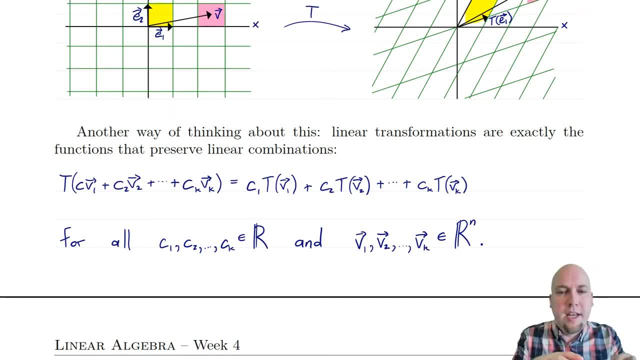 exactly the functions that sort of preserve linear combinations. They're exactly the functions that you can pull linear combinations out of. Okay, so in other words, they're exactly the functions with the property that t of linear combination equals that same linear combination, except with t applied. 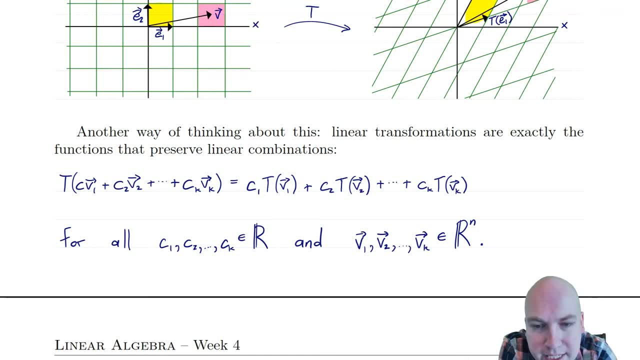 to each of the vectors individually. now, Right, so I've just sort of pulled each of the c's out and each of the sums out, Okay, and I've applied t to each of the vectors on the inside here, Okay, and sort of split it up. 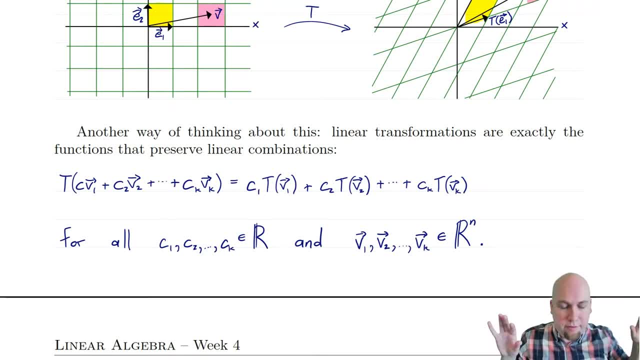 As much as possible. for most functions, you can't do that. Okay. for most functions, this is not a true equality. but for linear linear transformations or special linear transformations, this is true, Okay, no matter what scalars you pick and no matter what vectors you pick. 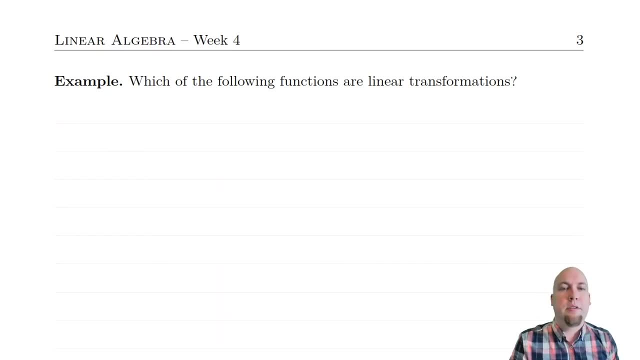 All right, so let's go through a couple examples. Let's actually see some linear transformations. So which of the following functions are linear transformations? So first example: suppose you've got some matrix. Okay, so I give you some matrix. It's an m by n matrix. Then I can define a. 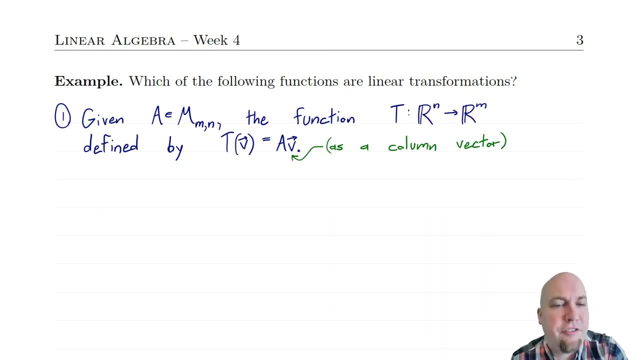 function based on this matrix. So I can define a function based on this matrix. I can define a function based on this matrix, And what I'm going to do is I'm going to define a function just via matrix. vector multiplication: Okay, so I'm going to think of my input, vector v. 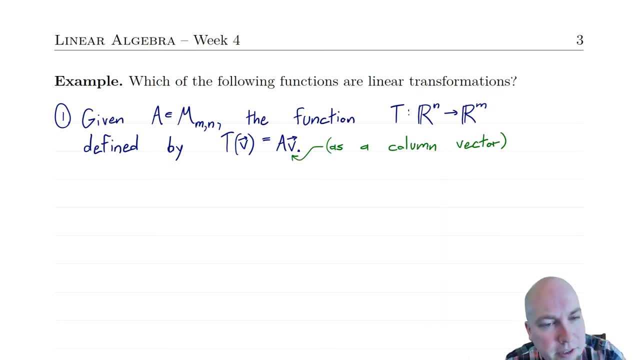 as a column vector, and then I'm just going to take that column vector and multiply it by some fixed matrix, a that's given to me. Okay, and when I do that? well, if I'm thinking of v as my input n-dimensional vector as a column, then this is going to be an. 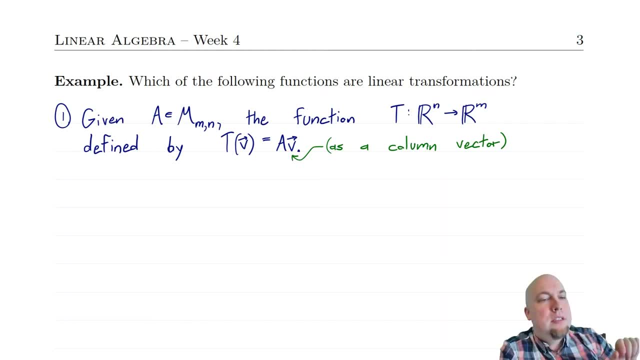 m by n times an n by one. Okay, so at the end of the day, I'm going to get an m by one column vector. I do this matrix multiplication. Okay, so I'm going to get something in m dimensions after I do. 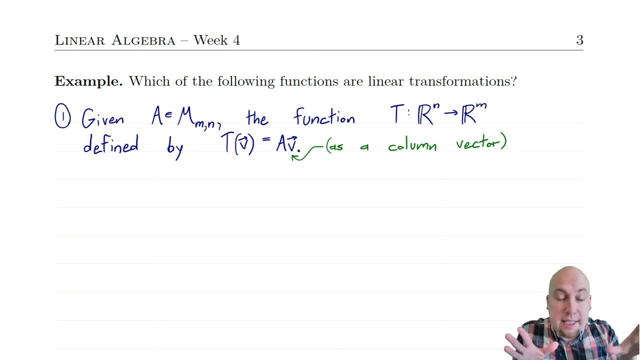 this. Okay, and then the question is: yeah, certainly this is a function, right, It's a rule for sending n-dimensional vectors to m-dimensional vectors. but is it a linear combination or, sorry, is it a linear transformation? Does it satisfy those extra two properties? Okay, so those properties that we 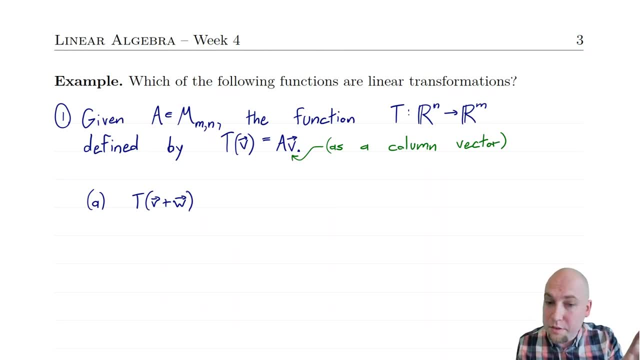 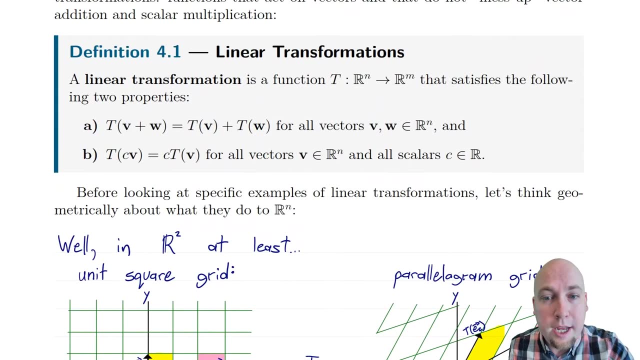 call a and b in the definition of a linear transformation. So let's check those. Okay, so let's check property a to start with. So I'm just going to scroll back up, remind you about what property a was. Property a was: well, does t of v plus w equal t of v plus t of w? Okay, well, 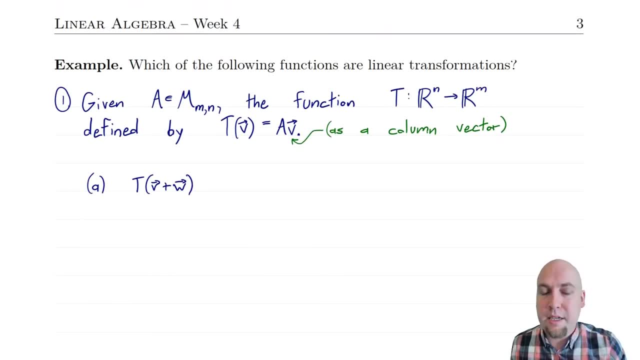 let's check that, Okay. so I start off with t of v plus w and I want to show that this equals t of v plus t of w. Okay, well, I mean t of v plus w, just by definition. just plug in the definition of your. 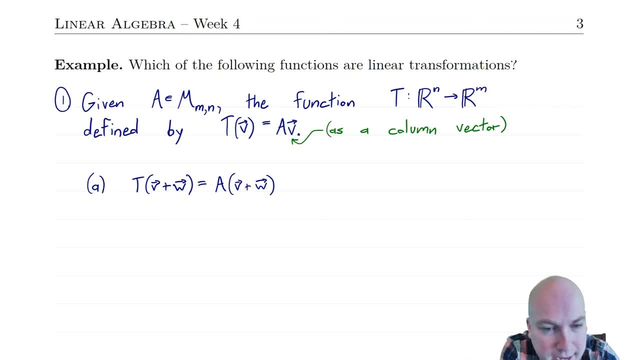 linear transformation. and well, t of v plus w equals a times v plus w. Great, okay, but now what I can do is: I mean, this is a matrix multiplication, and last week I learned all sorts of things about matrix multiplication. I know all of the nice properties that it has and, in particular, it has left. 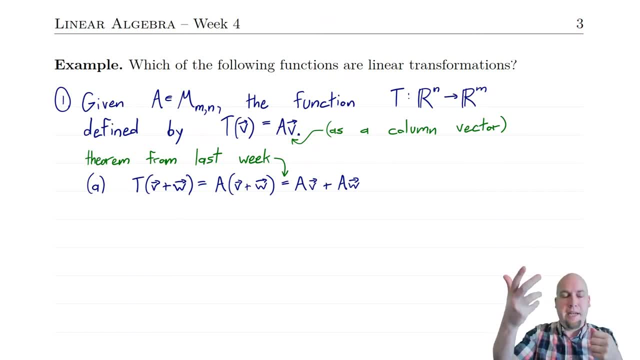 distributivity right. We had a theorem that said: ah yeah, if you have like a matrix a times b plus c, you can split that up as a b plus a c. Okay, so that's the theorem I'm using here, a theorem from: 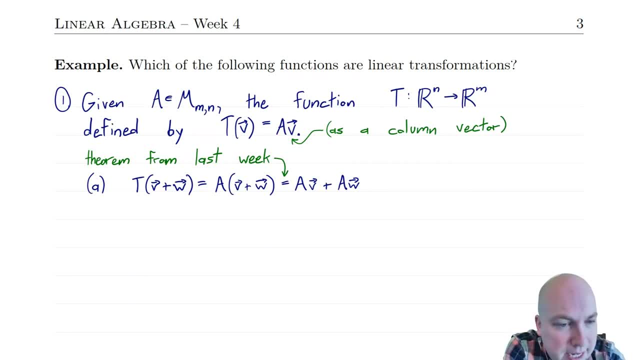 last week. I can split this up as a v plus a w, Okay. and now I just say: oh wait, a v, that's just t of v, And a w, that's just t of w. And that's exactly what I wanted. I've got t of v plus w, equals t of v. 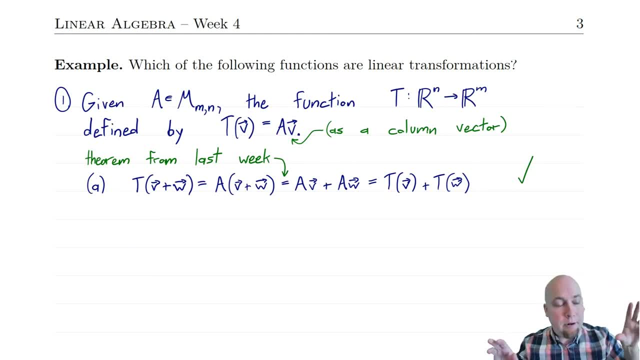 plus d of w. Great check mark because property a. now I see it's satisfied. Okay, so it's just using the definition everywhere and then using things that we know about matrix multiplication in the middle, All right. next to see the property b holds. we do the same thing with scalar. 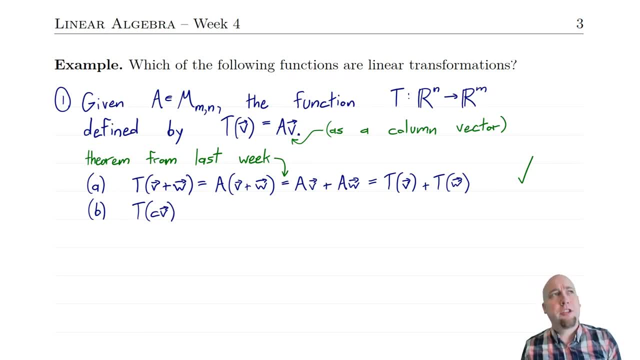 multiplication t of c times v. I want to show that that equals c times t of v. All right, so how do I? I do that? Well, again, I'm just going to use the definition and then things that I know about. 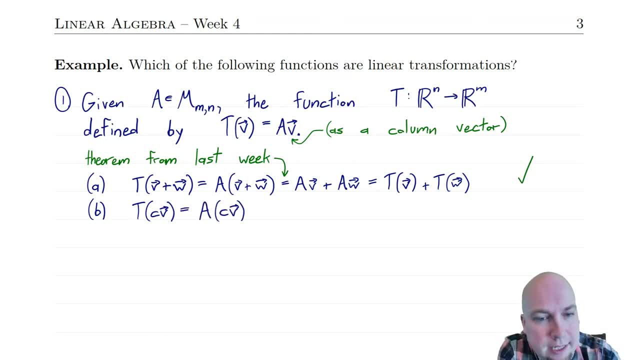 matrix multiplication. So start off with the definition of T. Well, T of CV equals A times CV. Okay, and now use things that you know about matrix multiplication And, in particular, the relevant thing that I know here is that if I have a matrix times a scalar times another matrix, 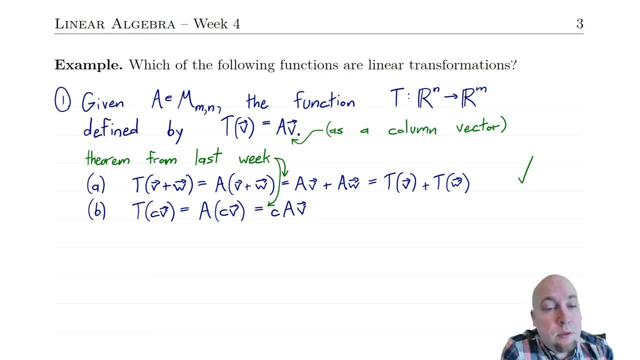 I can pull that scalar out in front, Okay. so again, this is just from a theorem from last week, one of our theorems that told us properties of matrix multiplication. Okay, and now AV. oh good, that's just T of V again, So I can substitute back in via the definition and I get exactly what I. 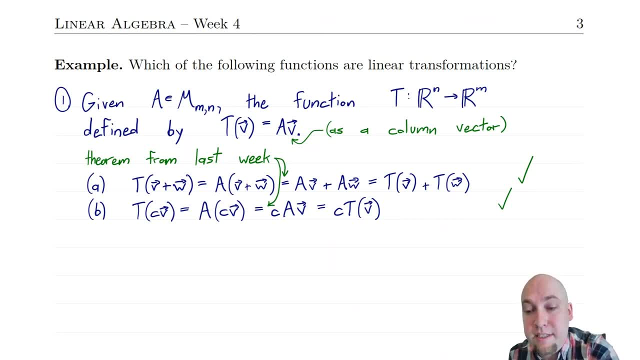 wanted. Okay, so property B of linear transformations is also satisfied. So then, because both of those properties, A and B, are satisfied, yes, T is a linear transformation, No matter what matrix you give me here. yeah, this function is a linear transformation. T of V equals A times B is a. 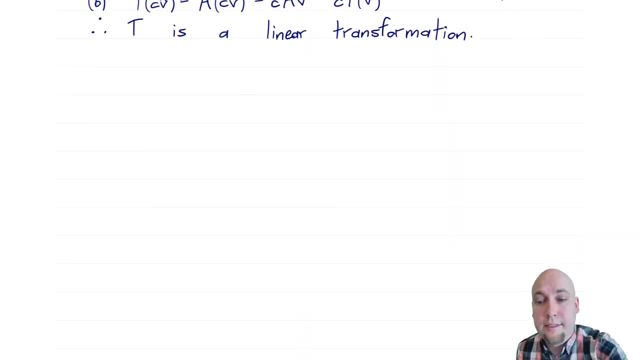 linear transformation. Great, All right. next up, how about this function that sends two-dimensional vectors to two-dimensional vectors via this formula here? Okay, so it sends the vector XY to X minus Y, X plus Y. All right, so let's show that this is a linear transformation as well. 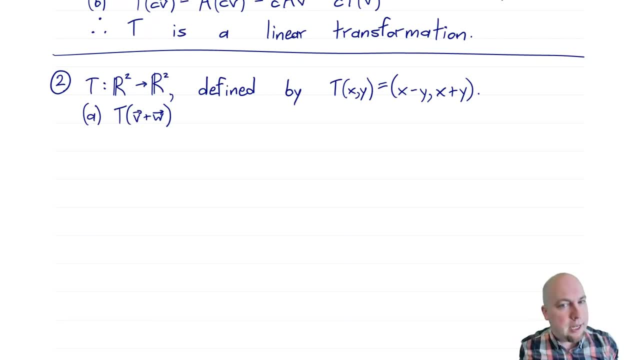 All right. so again, there are two things that you got to check. You've got to check that T of V plus W equals T of V plus T of W. You've got to check that T of CV equals C times C of V. Okay, 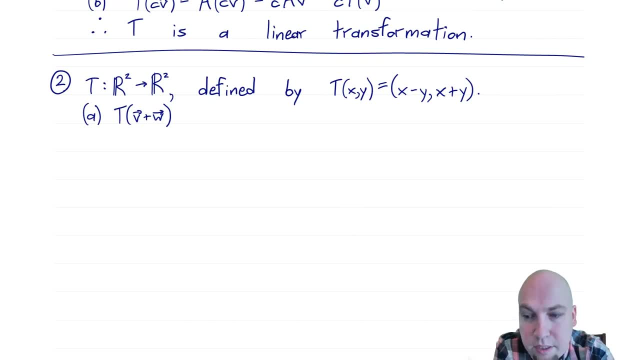 so it plays well with addition and scalar multiplication. So let's start off with addition And again just plug into the definition everywhere T of V plus W. Well, because this formula is defined in terms of the entries of the vector, I'm going to write this out a bit. 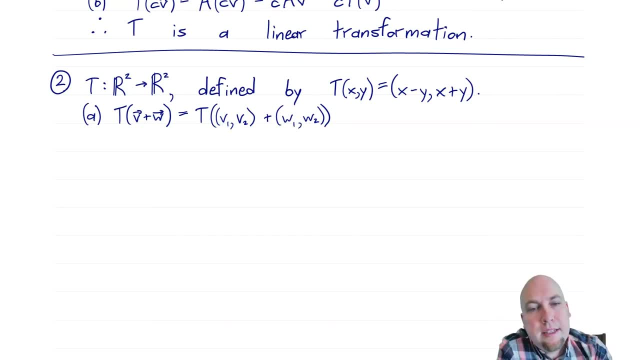 more explicitly in terms of the entries of the vectors. Okay, so V is V1, V2.. W is W1, W2.. Okay, and now I'm going to actually add those up. Okay, V1, V2 plus W1, W2. is this here First? 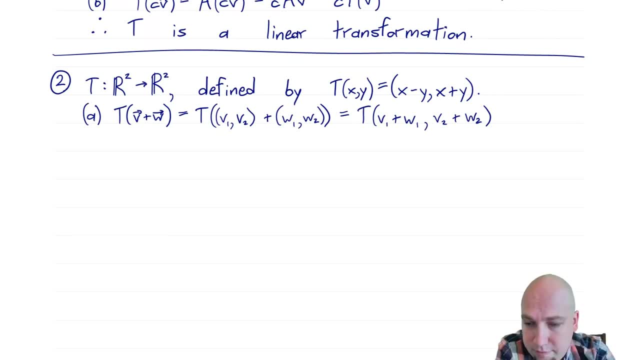 entry is just V1 plus W1.. Second entry is V2 plus W2.. Vector addition is just entry-wise. That's all I did there. And then this next step: now I'm using the definition of T right And the definition. 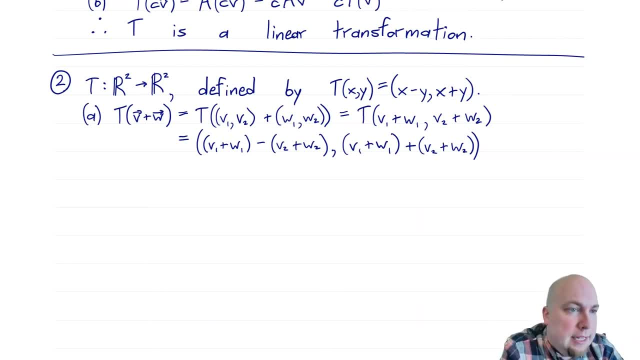 of T is. well, the output of T of something is just first entry minus second entry, and then first entry plus second entry. So that's all I'm doing here. I'm taking the first entry, V1 plus W1.. I'm subtracting the second input, V2 plus W2.. Okay, and that gives me my first output entry. 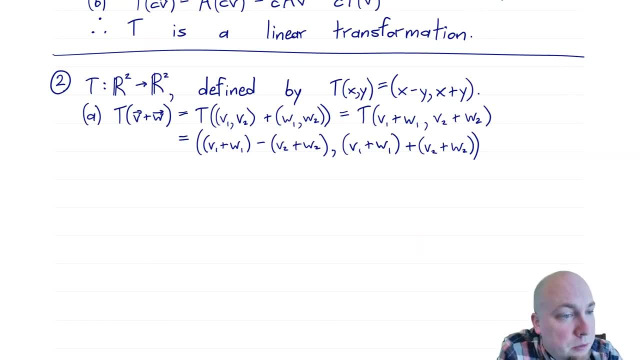 And then my second output entry is: just you sum up the two inputs, So V1 plus W1 plus V2 plus W2.. Okay, and I could probably simplify that a little bit and reduce it or whatever, but I'm just going to leave that there. And now what I'm going to do is I'm going to sort of work. 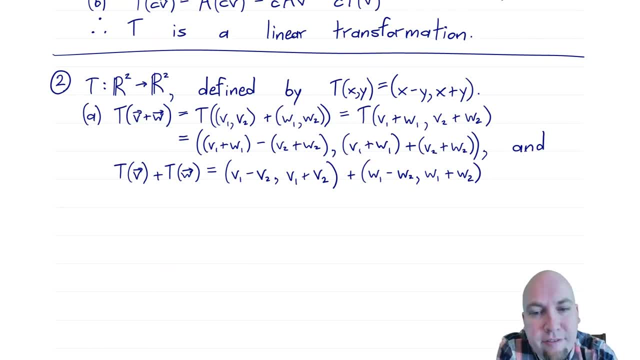 from the other side. I want to show that this equals T of V plus T of W. Well, let's just start with T of V plus T of W and see if we get the same thing after we simplify a bit. T of V. well, I mean. 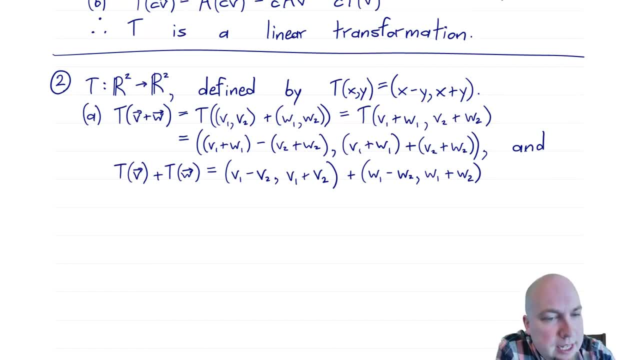 just use our formula here: It's V1 minus V2 in the first entry and V1 plus V2 in the second entry, And then T of W. same thing, except with Ws right: It's W1 minus W2 in the first entry, W1 plus W2 in the second entry. 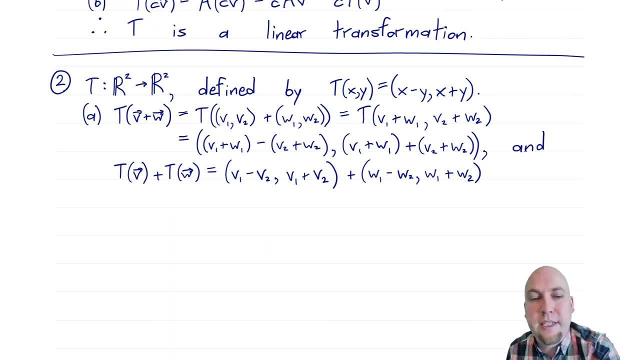 Okay, and now just use your definition of vector addition here and add things up. Okay, so just the sums of the first two entries: V1 minus V2 plus W1 minus W2.. Okay, and then: V1 plus V2 plus W1. 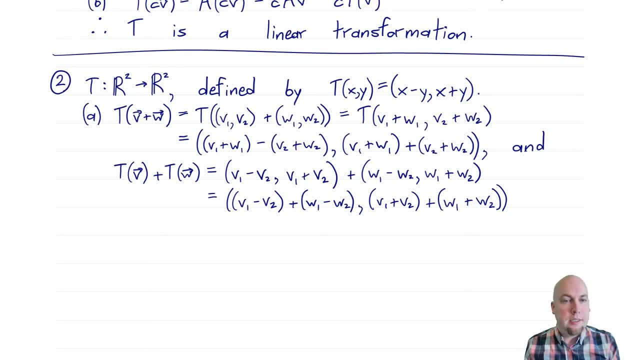 plus W2.. Okay, so just add things up. Okay, and then from here, all you do is you stare at things really hard. Okay, I want this to equal this And do those equal each other. Well, let's see, I've got a V1 here, a V1 here minus, V2 minus. 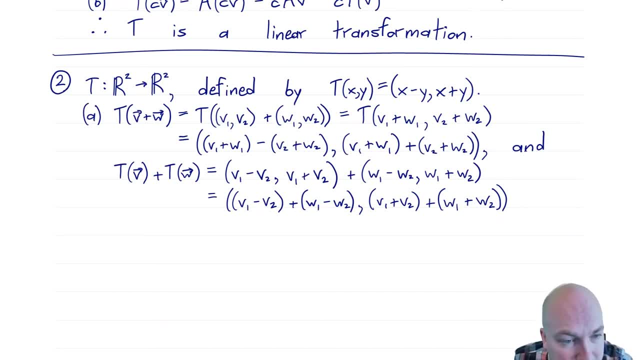 V2, a plus W1 plus W1, minus W2 minus W2.. Yeah, I mean, you just stare at it and match up all the terms. Yeah, every term that's down here is up here, and vice versa. Okay, they're the same thing. 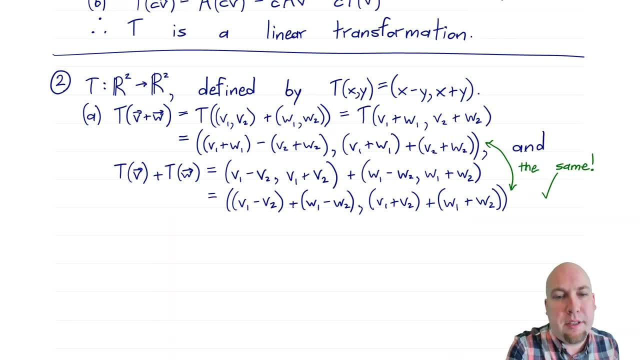 They're just written slightly differently. Okay, so those two vectors are the same. So, yay, we're happy. Property A holds All. right. now just do the same thing for property B. Show that you can pull scalar multiplication out of it as well. Again, just use the definition everywhere. Okay, T of C times V is well, okay. 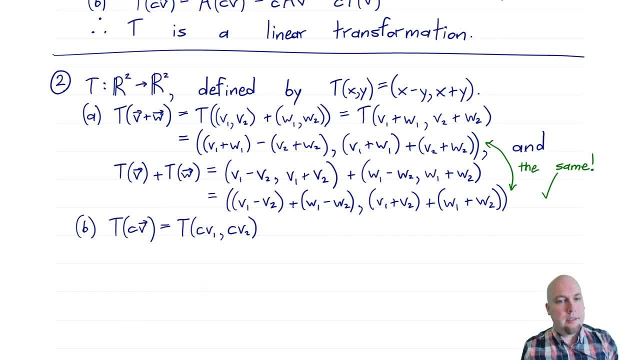 what is scalar multiplication? Well, you just multiply each of the entries by the scalar. Okay, so C of V1,, C of V2.. And then what is T of this? Well, just go back and use your definition of T. It's going to be first entry minus second entry, and then first entry plus second entry. 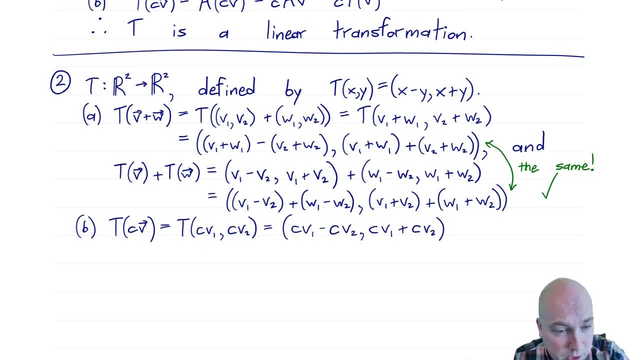 All right, so C of V1 minus C of V2, sorry, C of V1 minus C of V2, and then C of V1 plus C of V2.. Okay, I've just used the definition of T there, And now I just 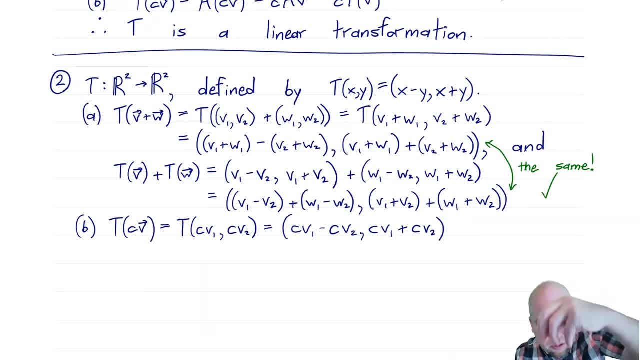 noticed that hey, there's a C in every single entry. there I can pull that out in front, because that's what scalar multiplication is right. So this is just C times V1 minus V2, V1 plus V2.. And then I look at this and I say, oh hey, great, That's just exactly what T of V1, V2 is. I just 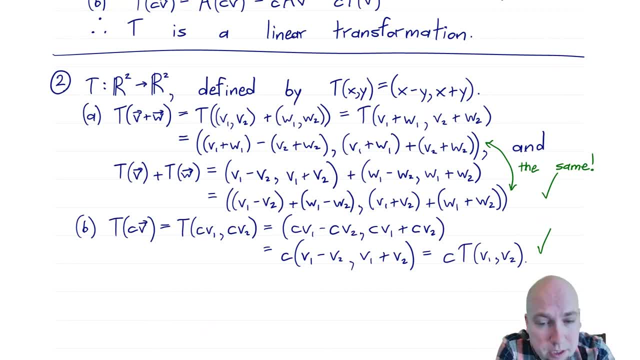 use my definition of T again. And then I'm done, because that's what I wanted to show. And now I've: C times V is the same as C times T of V. Okay, I can pull that scalar out. So great, because both of these properties are satisfied. that's a linear transformation as well. 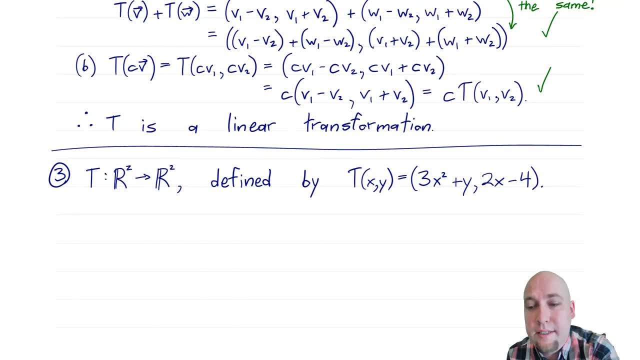 All right, let's do one last example here. This time it's a linear transformation from two dimensions to two dimensions again, but this time it's going to be defined by this weird formula here. So this time it's sending the vector XY to three times X squared plus Y, and then 2X minus. 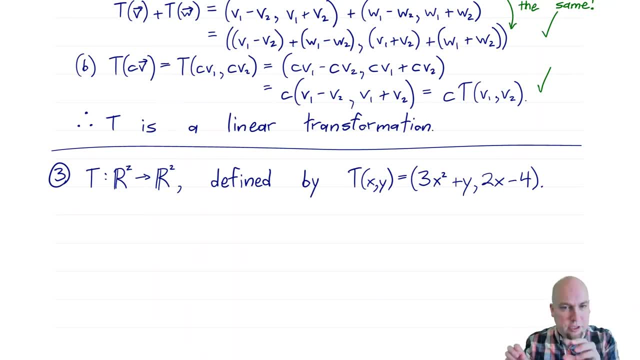 4.. So, again, this is a function. It's a function, It's a rule for sending two-dimensional vectors to two-dimensional vectors. The question is, is it a linear transformation? Does it satisfy those two extra properties that basically say that it's nice, say that it's something that we can study. 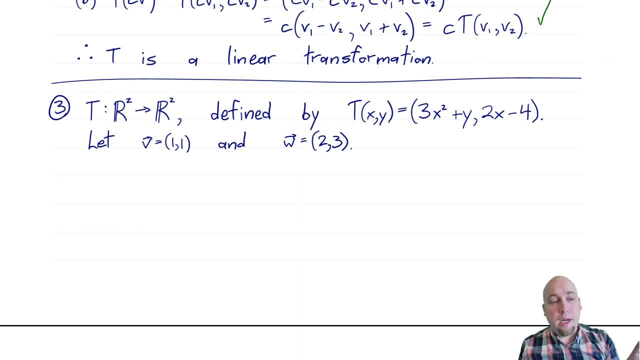 with linear algebra. Okay, and for this one I mean very naively, I just look at this X squared and that sort of makes me a little antsy, right, Because when I see that X squared I'm not thinking linear, That doesn't feel like a linear thing, right, That's a quadratic. 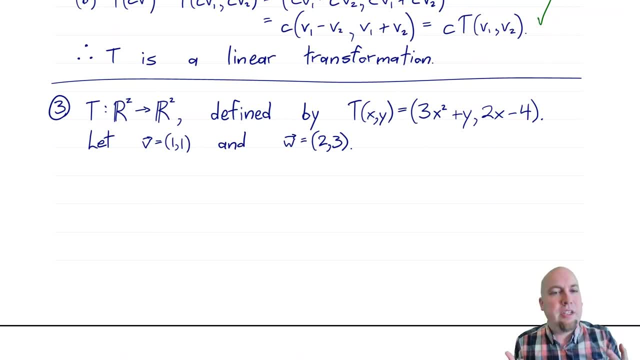 Graph, just X squared. that's a parabola. Okay. so it sort of doesn't feel linear. in a sense It feels like it's just violating the terminology linear transformation. So instead of trying to show that this is a linear transformation, I'm thinking it's probably not a linear transformation. 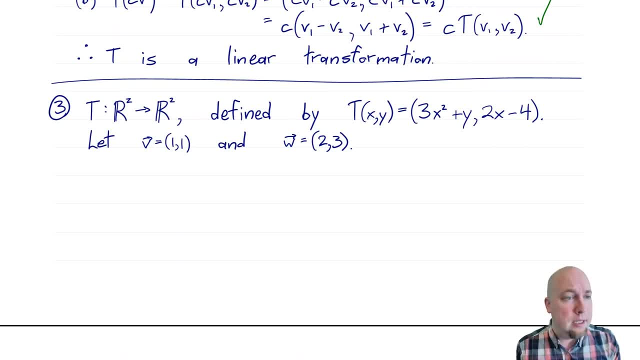 Let's show that it's not a linear transformation instead. Okay, let's really try to pin that down. Let's convince ourselves that that's true. Okay, so how do you show that something's not a linear transformation? Well, you have to show that at least one of the two defining properties 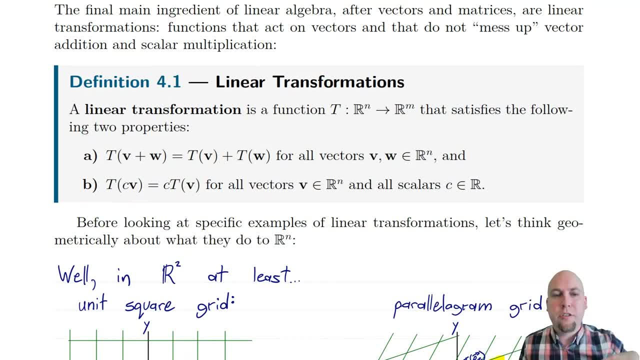 does not hold. So we go back to these two properties here, A and B. I want to show that at least one of them fails. Okay, so that just means I've got to find some particular counterexample for either property A or for property B. right, Like the opposite of A. 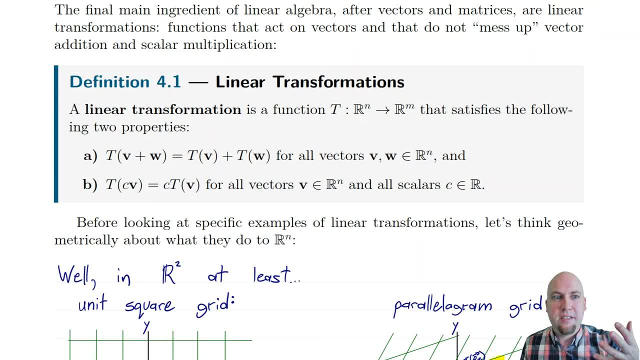 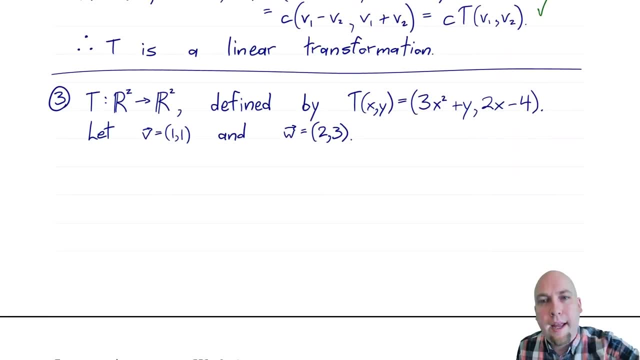 happens for all vectors is A. does not happen for some vector, Okay, so I've just got to find a particular counterexample. Okay, and it turns out. I mean, if you want to show that something's not a linear transformation, and you're trying to find a counterexample. 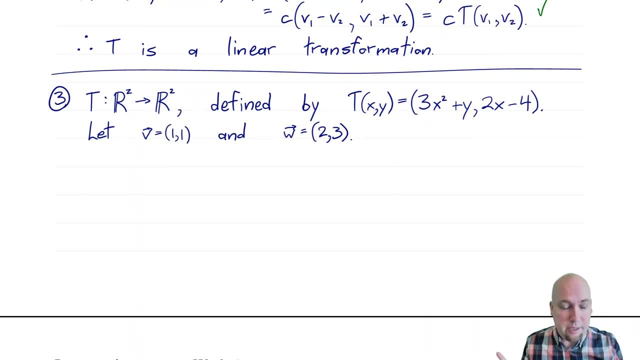 most of the time you can just pick them randomly, Okay, and you know, if there are counterexamples, they'll usually be very easy to find. So I'm just going to make up some vectors randomly here. Okay, V equals 1, 1 and W equals 2, 3.. Where did those come from? They came from just random places. 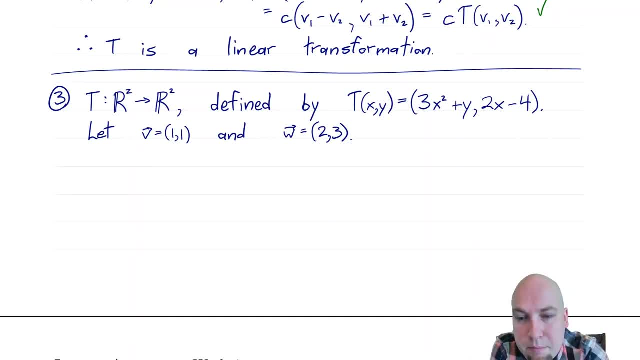 in my head: Okay, it does not matter where they came from. Okay, I made them up randomly And then I'm just going to check. you know, do the defining properties of a linear transformation hold for these two vectors? Okay, if they do hold, it tells me nothing, unfortunately, But if they, 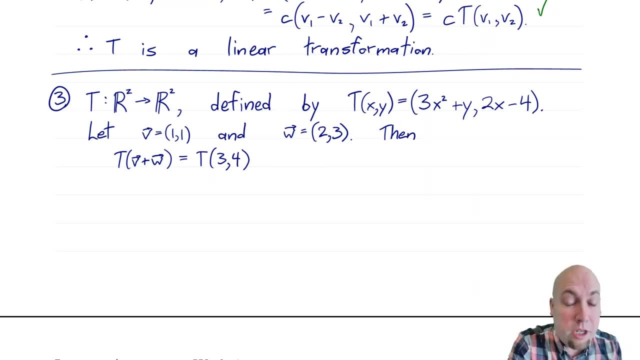 don't hold, then that's a counterexample that shows it's not a linear transformation. Not a linear transformation. All right. so T of V plus W. So for this one, what I've got to do is I've got to add V and W first. Okay. so 1, 1 plus 2, 3 is 3, 4.. So I want to do T of 3, 4.. Okay. 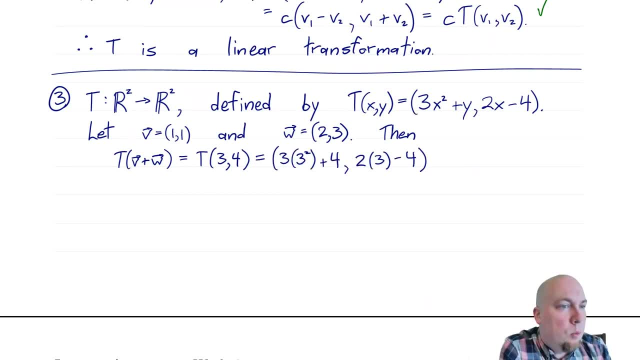 how do I do that? Well, I just plug into the definition: X is 3,, Y is 4.. All right, so it's just 3 times X squared. Well, that's 3 times 3 squared, And then plus Y, plus 4.. All right. 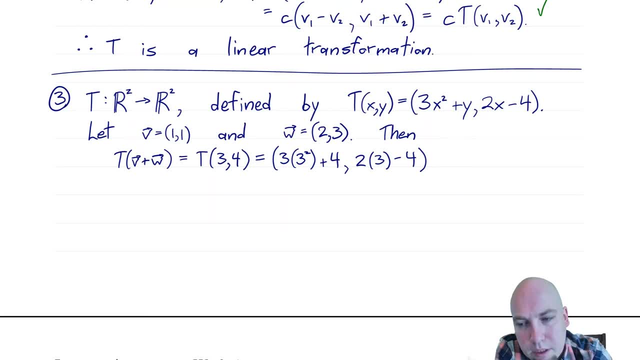 2 times X, that's 2 times 3 minus 4.. Okay, and I just compute those things, I get 31 in my first entry and 2 in my second entry. Great, Doesn't tell me anything yet, But now what I'm going to. 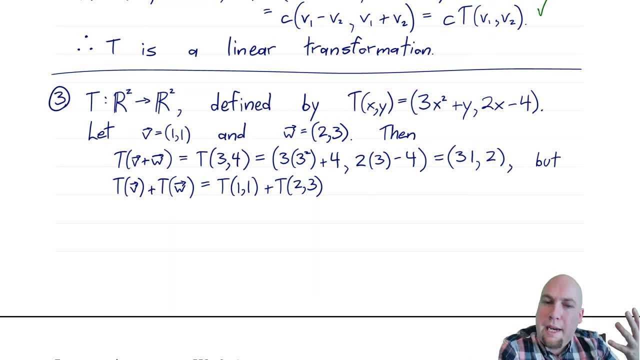 do is I'm going to compute T of V plus T of W and compare that, And my hope is that I get a different vector. If I get a different vector, then I know it's not a linear transformation. All right, so T of 1, 1 plus T of 2, 3, right, That's T of V plus T of W. Okay, and all I do is I plug these numbers. 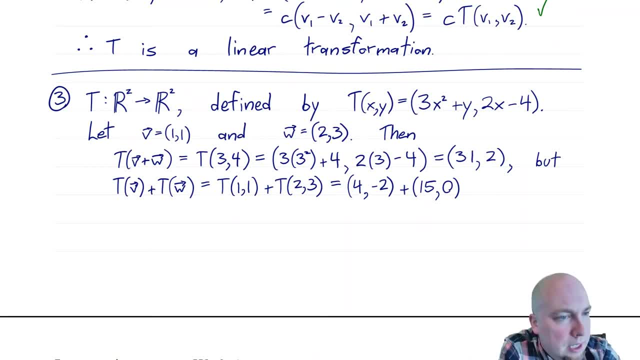 into the definition of T. So I plug 1, 1 in. So I'm going to get 3 plus 1 is 4 in the first entry, And then I'm going to get 2, minus 4 is minus 2 in the second entry. So that's T of 1, 1.. And then T of 2, 3.. Well, 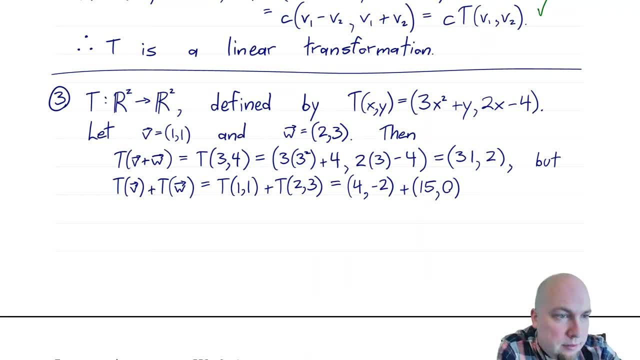 that's 3 times 2 squared, So that's 3 times 4.. That's 12.. Plus 3. Y is 3.. So that's 15 in the first entry, And then 2 times 2 is 4.. Minus 4 is 0 in the second entry. Okay, and then I add those. 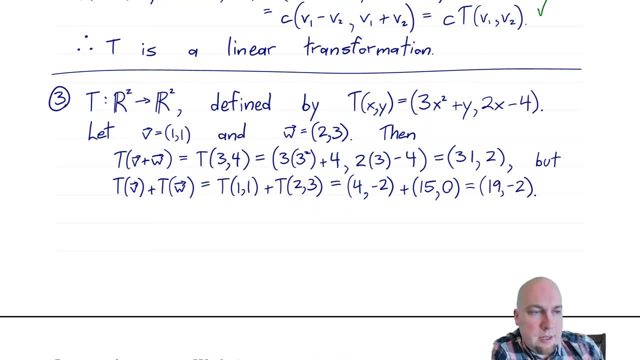 up And I'm going to get 19 and minus 2 as my answer here. And then I just look at these two vectors here And I ask myself: are those the same? And no, they're not the same, right, Okay? and because they're not the same, 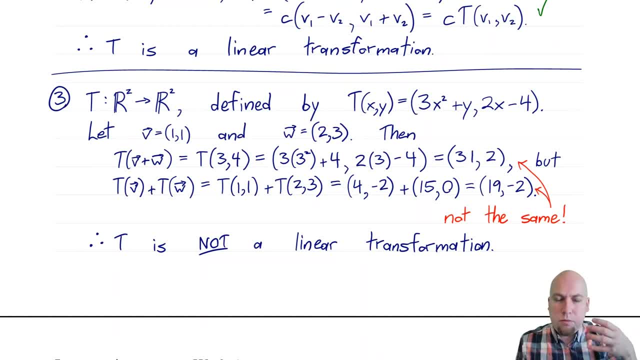 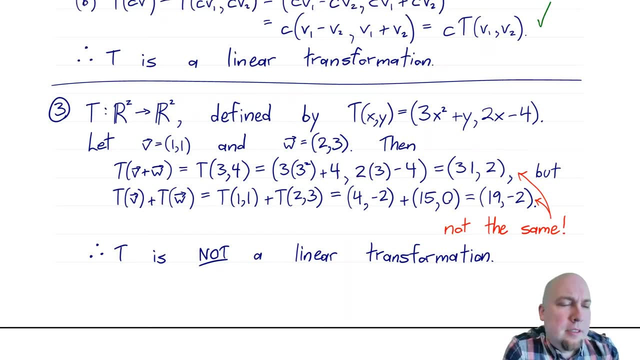 I know property A of linear transformations is violated. So no, like this is a function, but it's not a linear transformation. It's sort of not a nice function And, in particular, sort of what's going wrong with this function, What makes it not a linear? 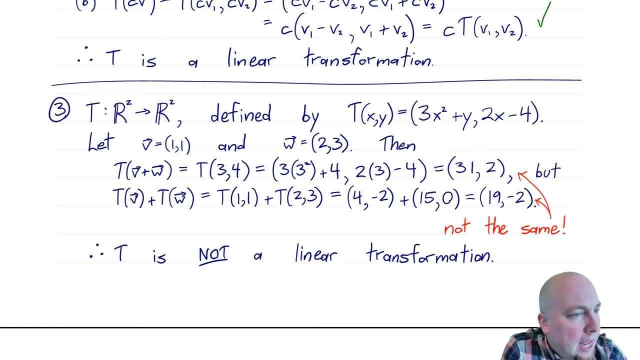 transformation is the fact that we've got a variable squared here And actually also the fact that we've got this minus 4 here. In a linear transformation you can only have scalars times, variables, And then additions and subtractions of those, So basically linear combinations of variables. 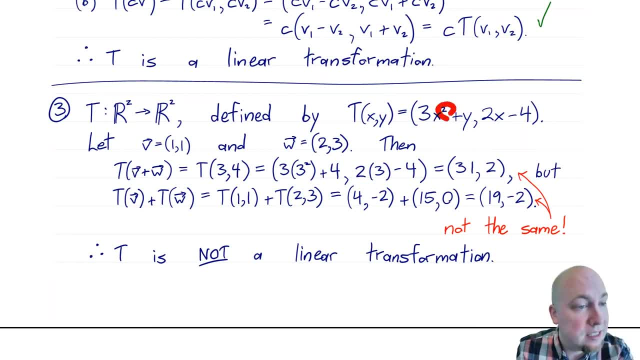 You can have things like 3x plus y, but not 3x squared plus y, Okay. and you can have things like 2x minus 4y, but not just 2x minus 4.. Both of those things cause problems. You also can't. 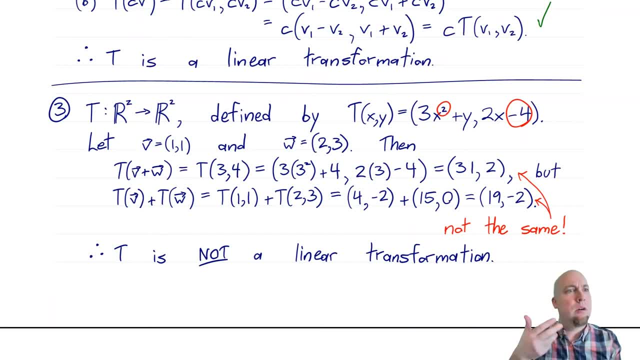 have things like x times y. You can't multiply variables, You can't do like cosine of x, You can't sort of do weird functions of variables. All of those things are disallowed. You can only do, you know, scalar times variable plus scalar times variable, and so on. 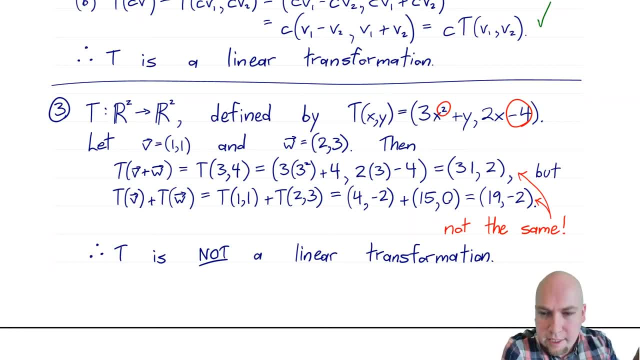 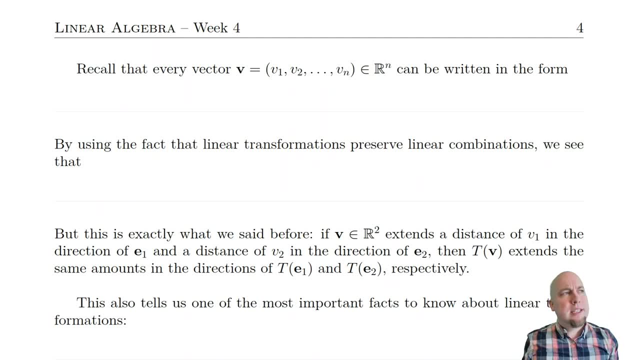 in each of the entries of the output, And that's something that we'll prove in the next lecture. Okay, so now what we're going to do to round out this lecture is: I'm going to go back and I'm going to try to convince you that that geometric interpretation of linear transformations, that 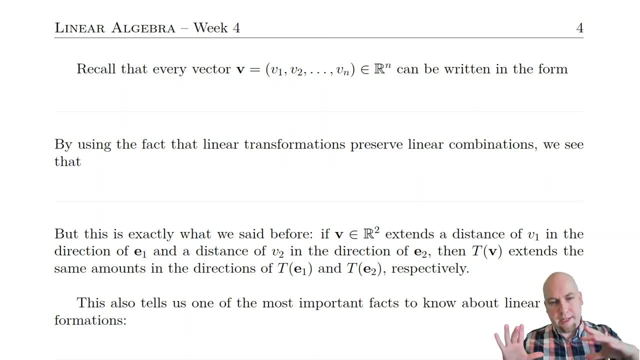 we talked about earlier. I'm going to try to convince you that that's true. So that picture where we had a square grid get turned into a parallelogram grid. Okay, and the way that this works, the way I'm going to try to convince you of that, is remember that every single vector can be. 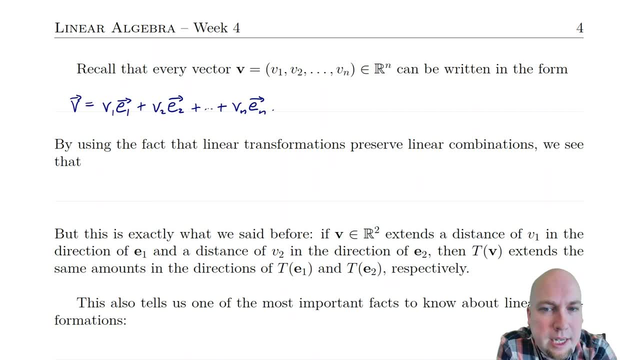 written as a linear combination of the linear transformation, of the linear transformation of the standard basis vectors. So you can write it as you know: first entry of v times e1 plus second entry of v times e2, all the way up to the last entry of v times en. where remember these e? 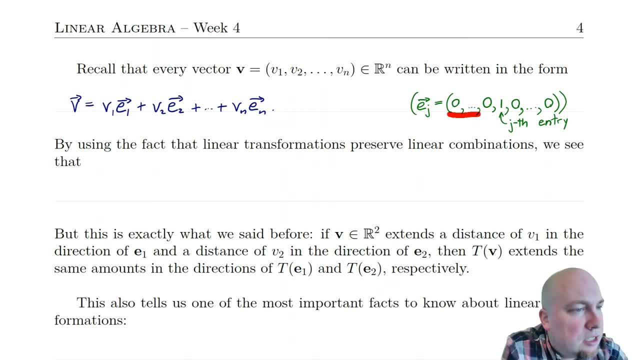 vectors, these standard basis vectors. those are the vectors that have just a single one in one of their entries and everywhere else is zero. Okay, so well, if we use this fact together with the fact that linear transformations are the functions that preserve linear transformations? 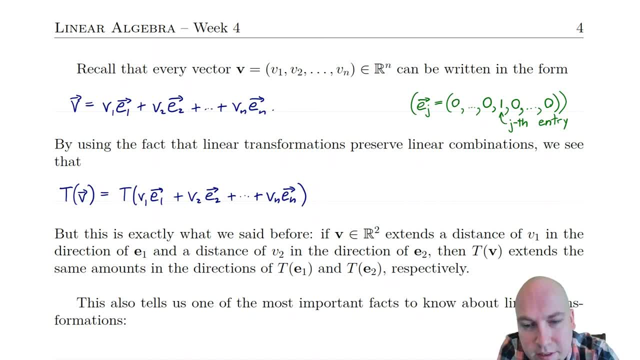 then what we get is: well, t of some vector is t of this linear combination up here, and now we split it up because t is a linear transformation. then what we get is: t of v equals its first entry times, t of e1 plus its. 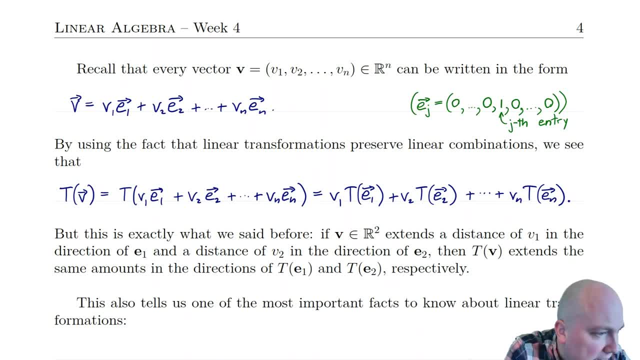 second entry times t of e2 all the way up to its last entry times t of en. Okay, and at first this just looks like a mess of symbols, but what this tells us is very important. This tells us this equation right here encapsulates the fact that unit square grid gets 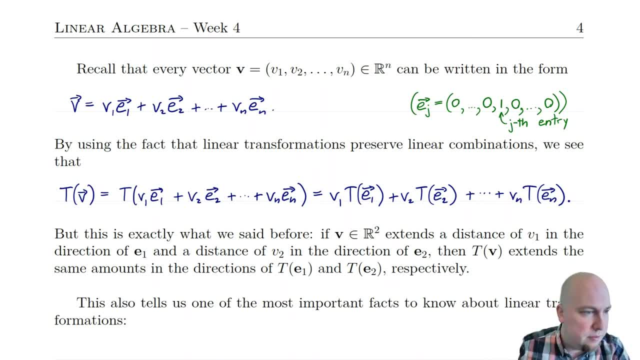 gets sent to parallelogram grid because, for example, in the two-dimensional case- so if n is two and the sum doesn't have this junk over here, it just has the first two entries- then what this is saying is: t of v is sent to the vector that points v1 units in the direction of t of e1, and 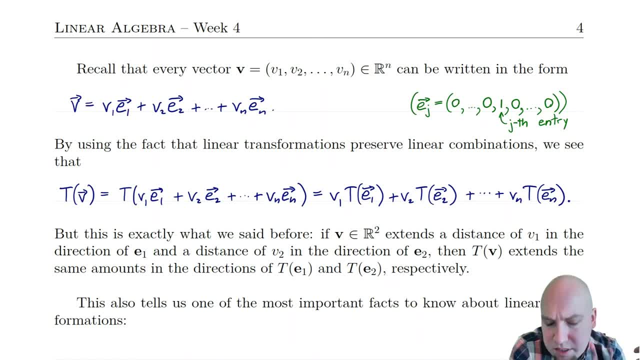 v2 units in the direction of t of e2, whereas it used to be the vector that pointed v1 units in the direction of e1 and v2 units in the direction of e2.. So all that happened, like it's still sort. 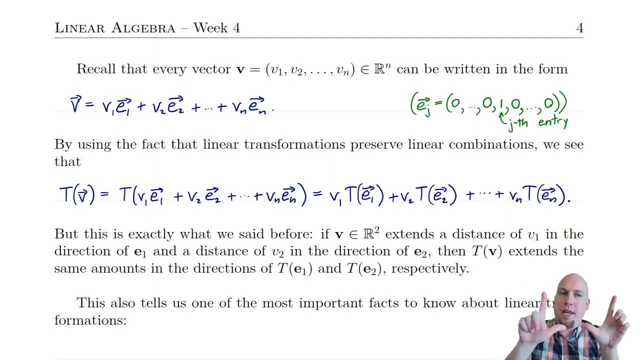 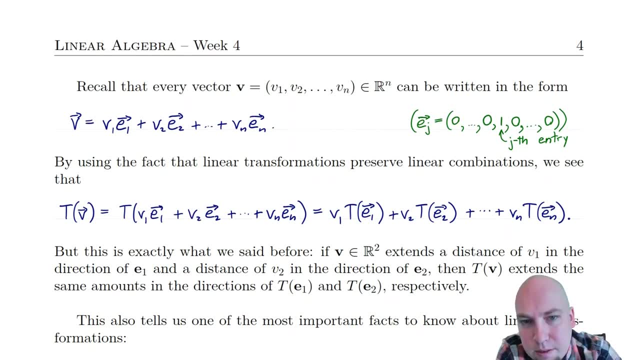 of pointing the same amount in these two directions. all that's changed is, you know, the those two directions changed. It's no longer e1 and e2, now it's t of e1 and t of e2.. Okay, so again, let's go back, show you that picture to try to sort of pin this down again. Okay, 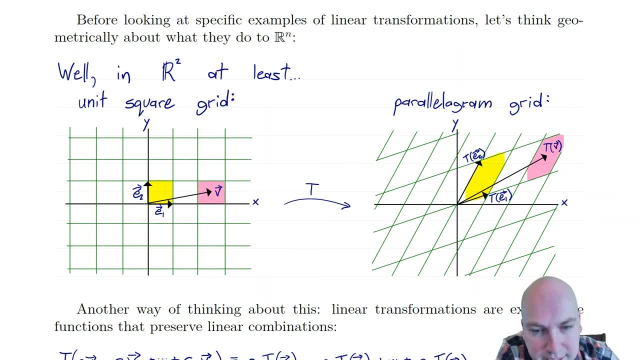 so v it used to point you know some amount in the e1 direction and some amount in the e2 direction. Now it points those same amounts in the t of e1 and t of e2 directions instead. So now, instead of pointing over, you know 2.5 boxes that way and half a box up, now it points. 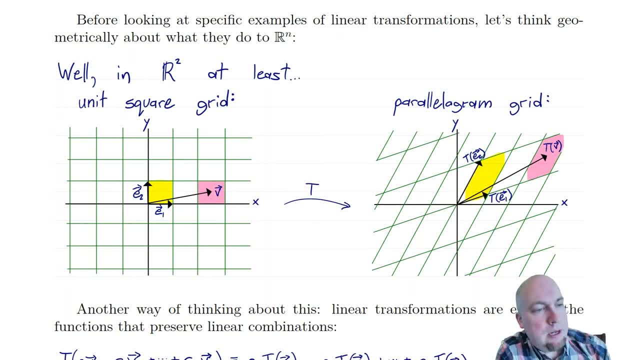 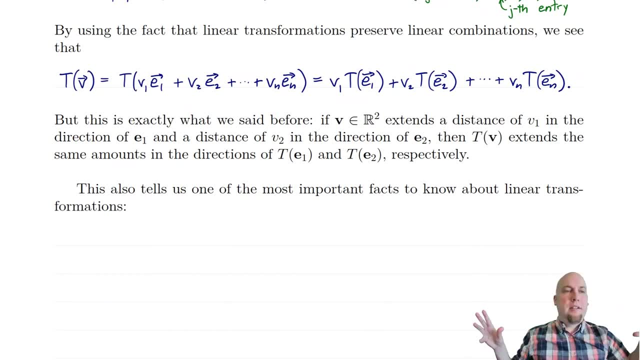 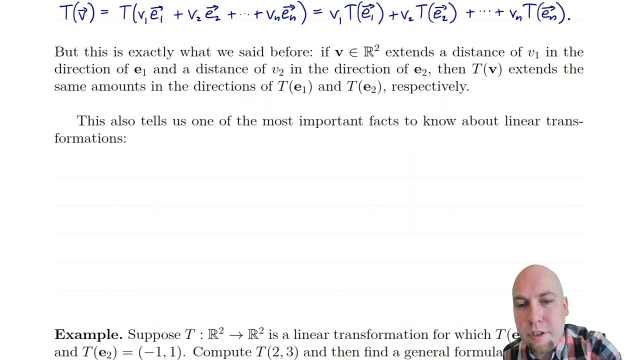 0.5 parallelograms this way and 0.5 parallelograms up that way. Okay, so, in other words, everything's spread sort of uniformly out by this function here, by this linear transformation. Another way of saying this is linear transformations. 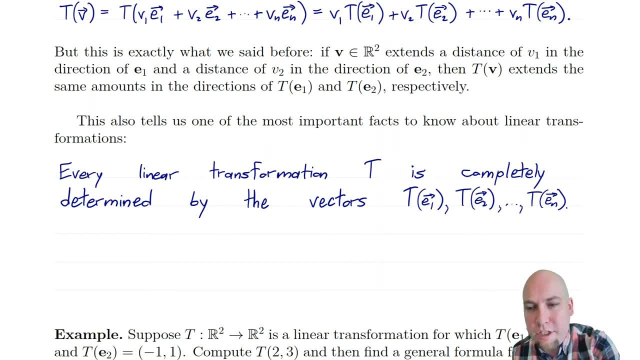 they have the remarkable property that they're completely determined by n vectors. okay, They're completely determined by t of e1 and t of e2, all the way up to t of e, n. If you know what a linear transformation does to this vector, then you know that it's a linear transformation. So 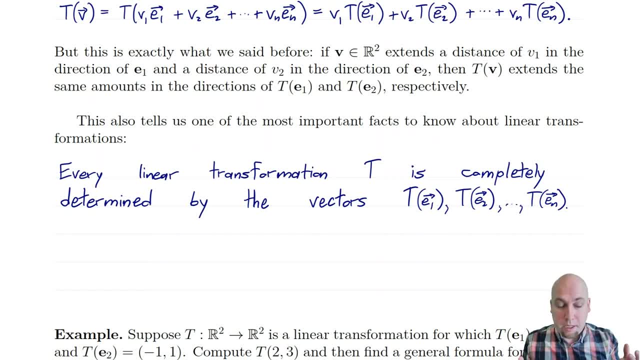 if you know what a linear transformation does to the standard basis vectors, then actually, very remarkably, you know what they do to every single vector. That's enough to completely reconstruct the linear transformation. the entire function okay, And this is very, very different. 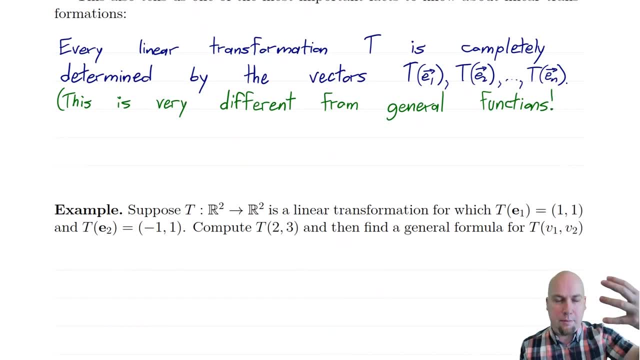 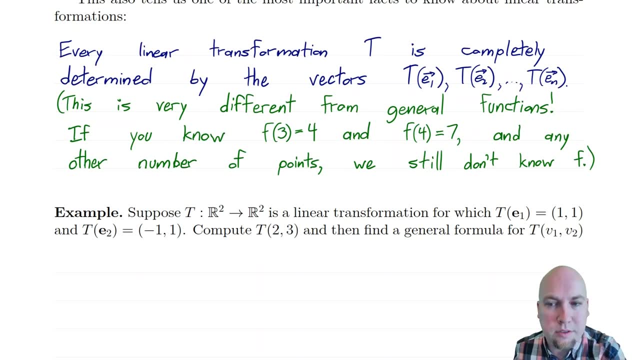 from functions in general, even functions of just one variable, of just a single real number. right, If you have a function of a real number, and let's say that you know that you know f of 3 equals 4, and let's say that you also know f of 4 equals 7, and maybe you know a whole bunch of. 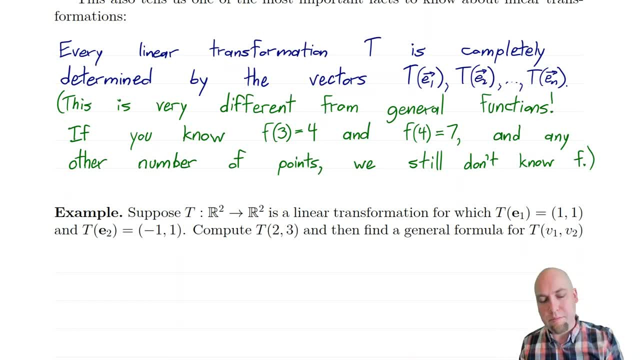 points. okay, You know, f of 5 equals 19,, and f of 6 equals minus 3, and f of 7 equals 48,. okay, And that finite list is however long you like. Well, you still don't know what f is. 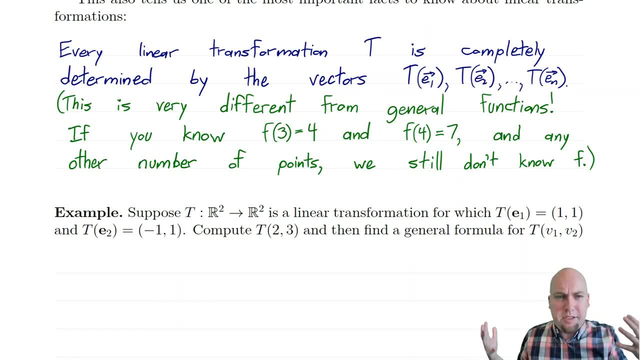 okay, No matter how many individual data points you have, you still don't know what the actual function is because, like you can find polynomials that go through whatever points you like, and you can find infinitely many, even just polynomials that go through any finite number- 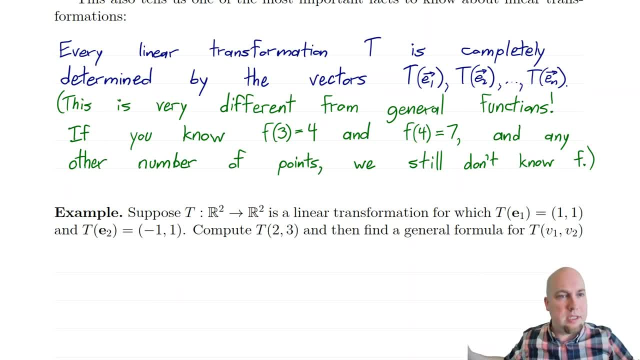 of points that you like, never mind even more exotic functions like cosine and sine and logarithms and exponentials, And functions that are even worse than that, things that aren't even differentiable. okay, So linear transformations: they're really remarkable. You just need a finite amount of data. 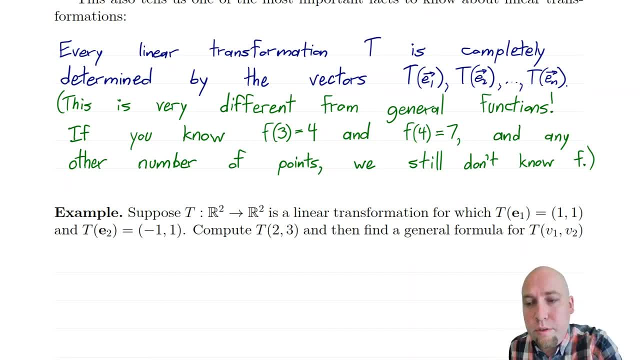 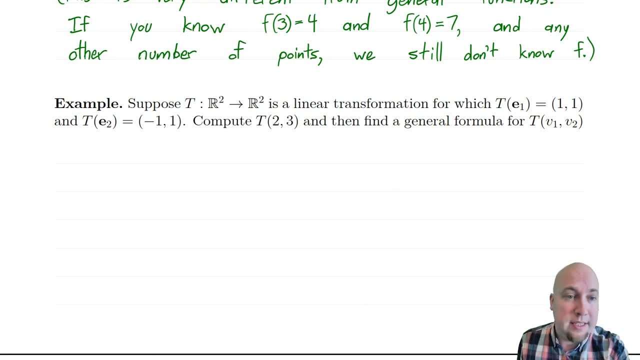 to reconstruct the entire function. all right, Let's go through one example of how to actually do this. okay, So suppose we've got a function and we're told two things: We're told that it's a linear transformation and we're told what it does to the standard basis vectors. okay, Well, 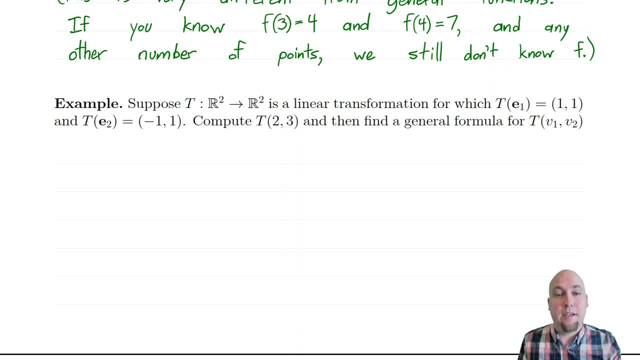 if you have those pieces of information, you can reconstruct it entirely. So what we're going to do is, based on these two data points- T of E1 and T of E2, we're going to figure out what T of 2,3 is. 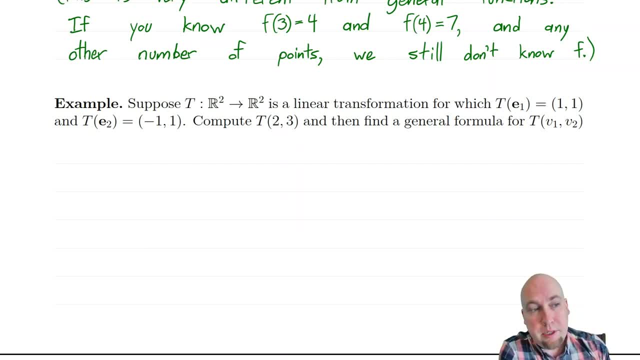 and we're also going to construct a general formula for that linear transformation. So we're going to be able to compute T of V1, V2, no matter what V1 and V2 are, All right, but let's start off with T of 2,3, just to see how it works. all right. And the trick is write 2,3 as a linear combination. 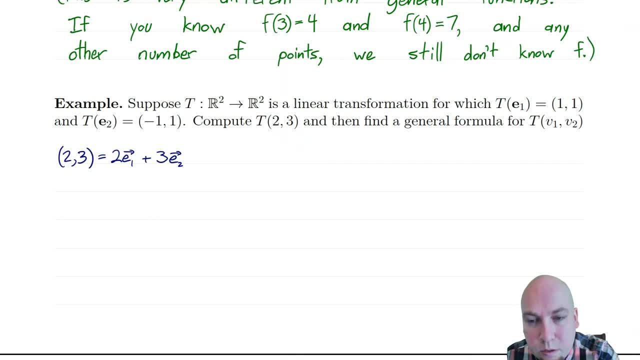 of those standard basis vectors. okay, And we saw how to do this earlier in the course. 2,3 is well, you just peel off those coefficients, It's 2 times the first standard basis vector plus 3 times the second standard basis vector. all right, And then you apply T to it. okay, T of 2,3. 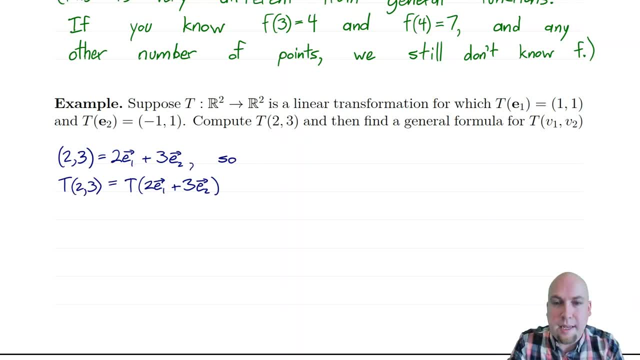 is T of this linear combination, because those are the same thing. okay, And now use the fact that it's a linear transformation. Use the fact that T is a linear transformation to split that up. okay, T of junk is 2 times T of E1 plus 3 times T of E2, okay, So we just brought. 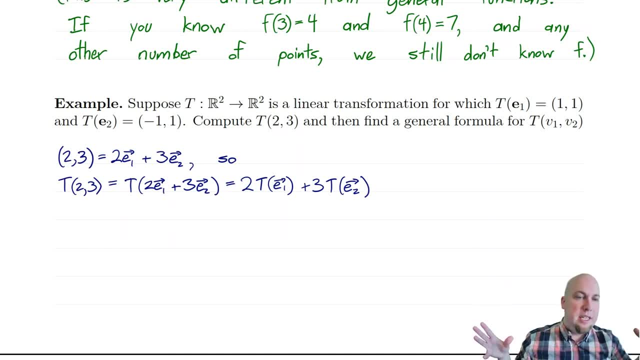 the twos and the vector addition outside of T, because it's a linear transformation, so we can't do that. okay, and now, hey, t of e1. i know what that is. the question told me. t of e1 is the vector 1, 1. 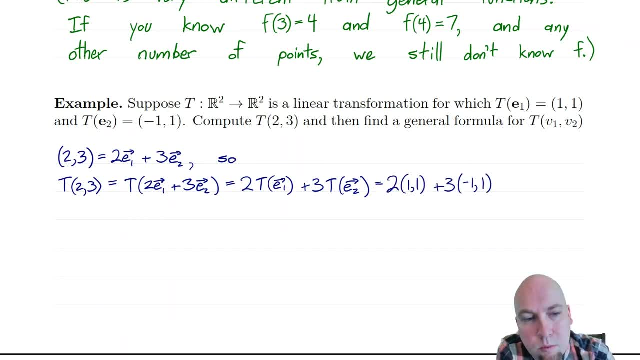 and t of e2- again, i know what that is. that's the vector minus 1- 1. okay. so just make those substitutions. and now it's just scalar multiply and add them all up and at the end of the day you're going to get the vector minus 1- 5, okay. so if you ever have any linear transformation, that 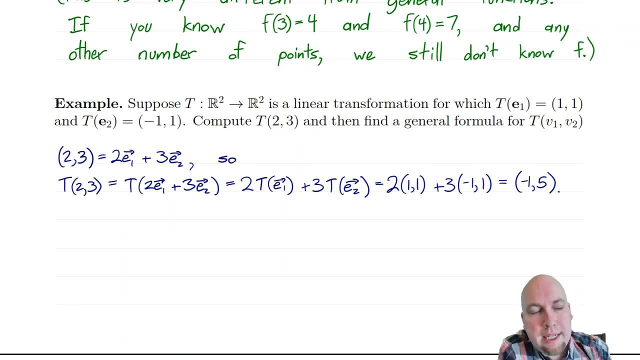 sends e1 to 1: 1 and e2 to minus 1: 1, then it must send the vector 2: 3 to minus 1: 5. okay, there's no other possibility, or else it can't be a linear transformation. like it'll still be a function. 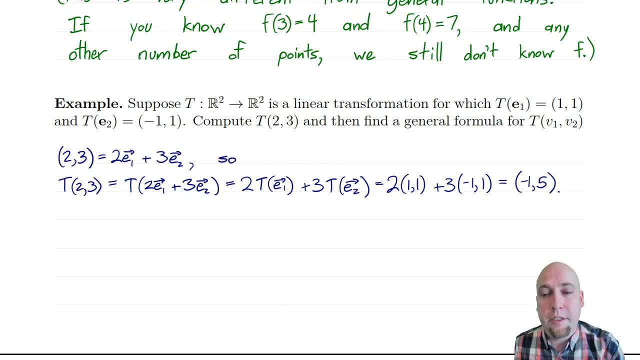 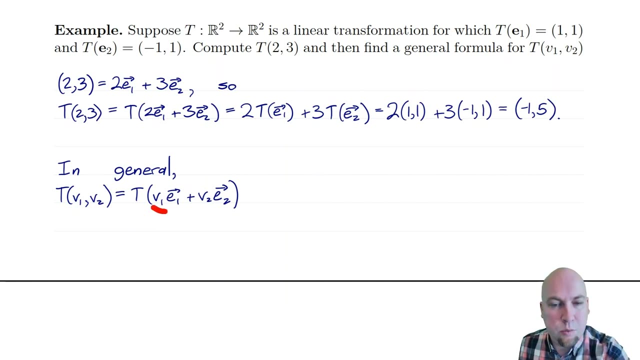 if it sends 2, 3 somewhere else, but it won't be a linear transformation, all right. so let's generalize this a little bit and figure out an explicit formula for t of v1- v2. okay, so slightly more generally, if you have t of v1- v2, well, you can write v1- v2 as v1 times e1 plus v2 times e2. 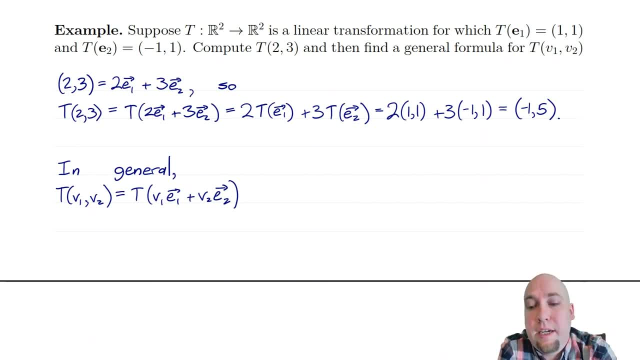 so just write that vector as a linear combination of the standard basis vectors and then split that linear combination up and then you can write that vector as a linear combination of the standard basis vector up again, because t is a linear transformation. so you can do that, okay. so this: 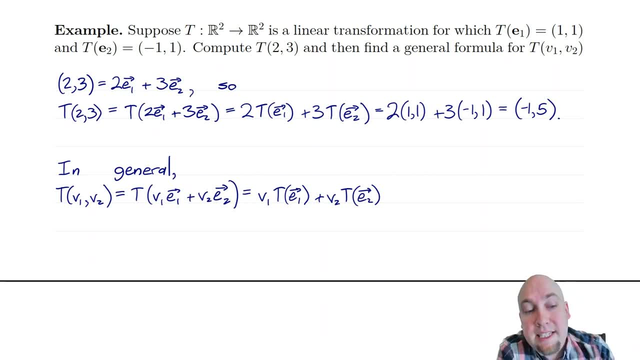 is v1 times t of v1 plus v2 times t of v2. okay, and then just sub in: what are these vectors here? what is t of v1? ah well, that's 1, 1, and what is t of v2? ah well, that's minus 1, 1. so just sub those. 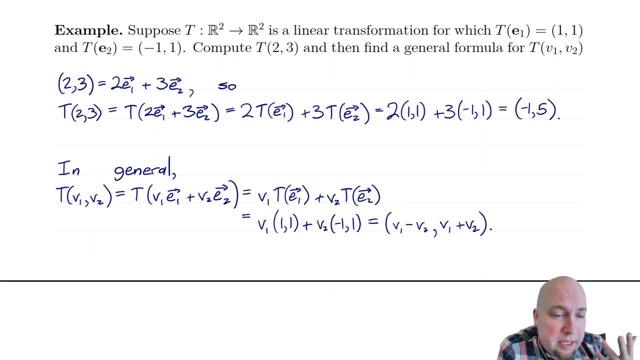 in there. you get this and then do the scalar multiplication and vectors vector addition and you find that t of v1- v2 must equal v1 minus v2, v1 plus v2. okay, and this is actually a linear transformation that we saw back a couple examples ago. so this is exactly this linear